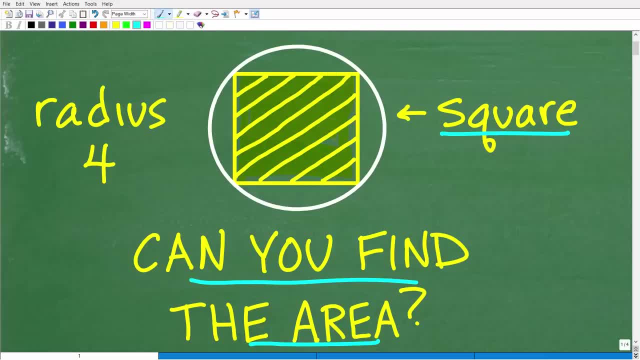 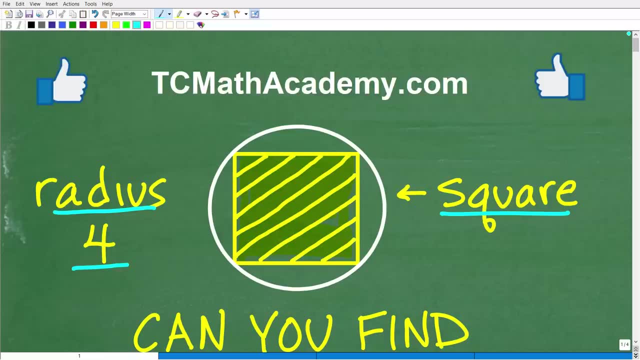 the corners are touching the actual circle And the only information that we have is that the radius of the circle is 4.. Okay, so that is the question, And feel free to use a calculator, But if you can figure this out, go ahead and put your answer into the comment section. 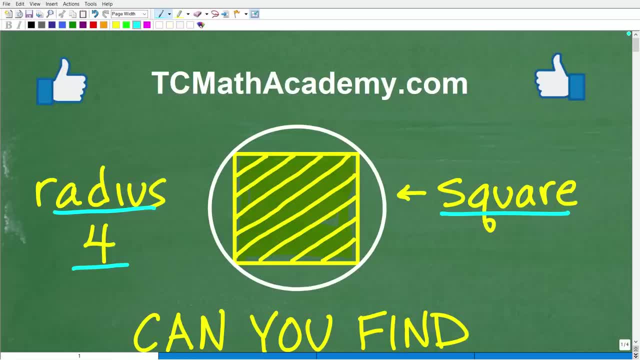 I'll show you the correct answer in just one second, And then, of course, I'm going to solve this interesting little geometry problem step by step. But before we get started, let me quickly introduce myself. My name is John, and I have been teaching middle and high school. 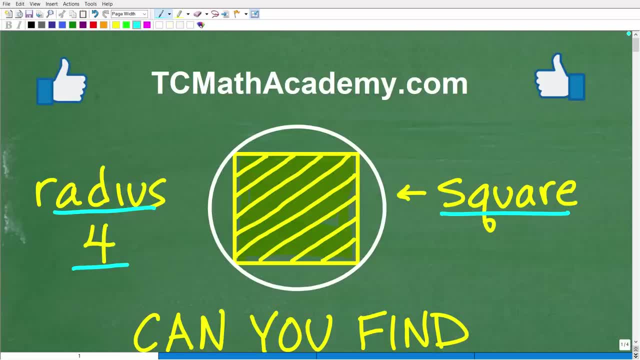 math for decades And it really is my true passion to try to make learning and learning math as easy as possible. So if you need assistance in mathematics, check out my math help program at tcmathacademycom. You can find a link to that in the description below, And if this video helps, 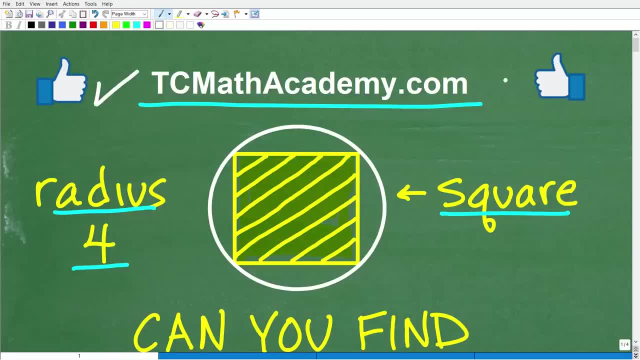 you out, or if you just enjoy this content, make sure to like and subscribe, as that definitely helps me out. Okay, so let's go ahead and take a look at the answer Again. we're trying to find the area of this square that's inscribed of this circle, And the only thing that we know is that 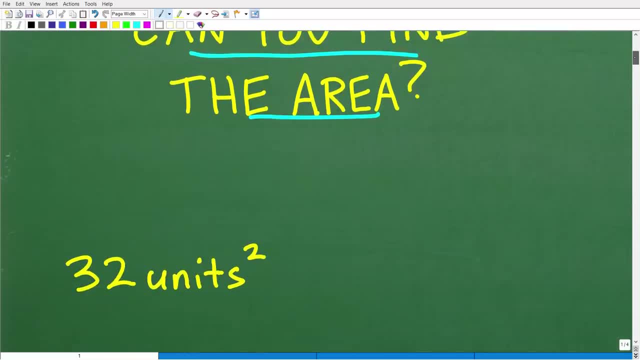 the radius of the circle is 4.. Well, the correct answer is 4.. So let's go ahead and take a look at the answer. The correct answer is 32 units squared. Okay. so how did you do? Well, if you got this, 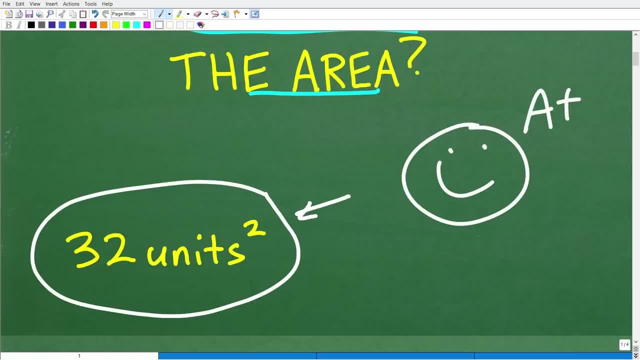 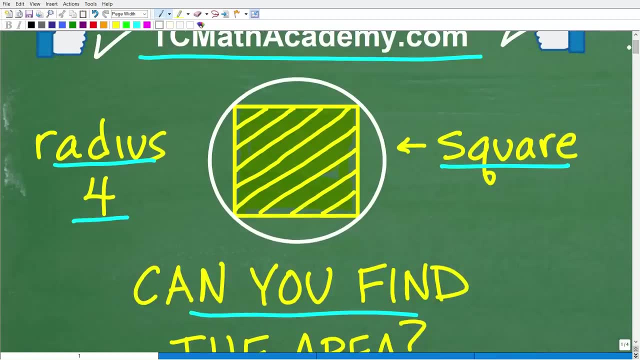 right, we have to celebrate by giving you a nice little happy face, an A+, a 100% and multiple stars, So you can brag to your friends and family that indeed you are a certified professional expert in the area of solving basic, interesting geometry problems. Now your friends and family. 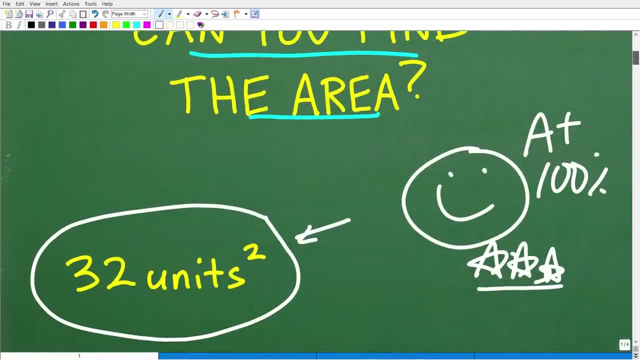 may not be that impressed, but you really should feel proud of yourself if you are able to solve this problem. So let's go ahead and take a look at the answer And if you got this right problem, And if you're kind of like lost here, if you're like, wow, I don't even know where to. 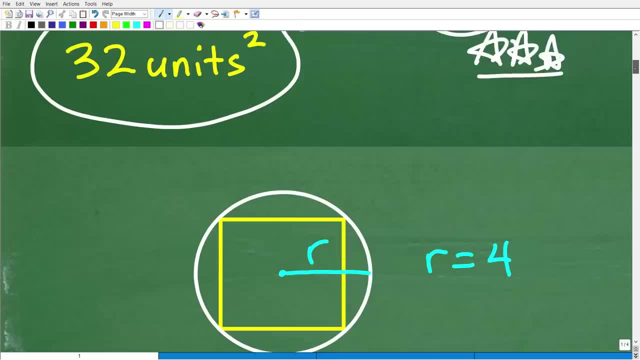 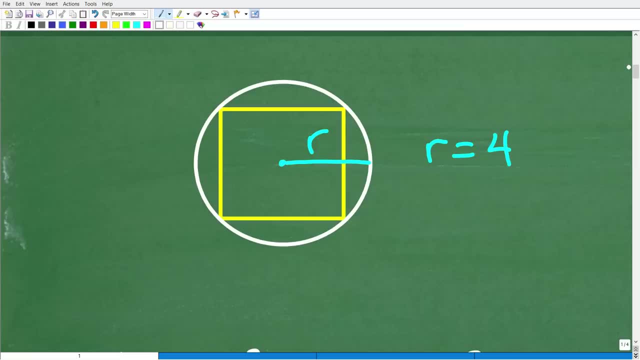 start. Well, I'm going to show you exactly where to start, So let's get into it. This is not that difficult, but you certainly need to know some basic, important concepts about circles and squares and triangles. I'll get to that in just one second. But here is effectively the problem. 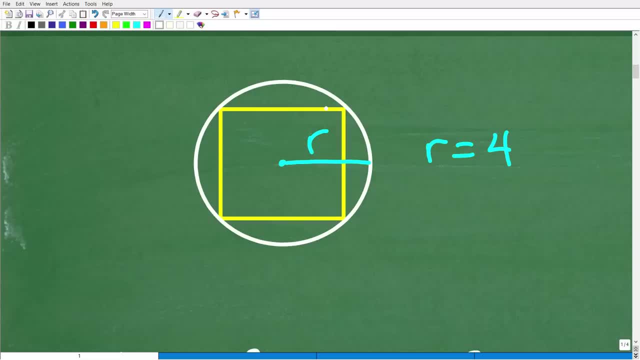 So we have this square inscribed inside of this circle. So, again, that means that this, uh, corners of the square are in fact touching the circle. Now, what do we know about squares? Well, we know that the sides are equal, right? So when you have a square, each side is equal to. 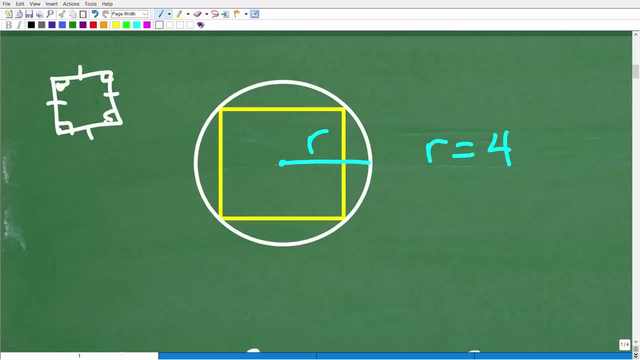 the other and the angles are 90 degrees. So, by definition, this is a square. So this circle. we do know that the circle's radius is four. Now, what is the radius of a circle? Well, you can see here: uh, this is the radius, right here It's of course, the radius is four. 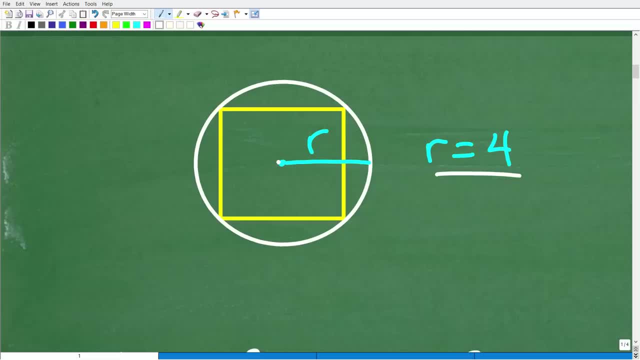 but the radius emanates from the center of the circle. So here, if I have a circle from the center, from the center out to any point on the circle, that is the radius And twice the radius is what we call the diameter. Okay, So you can see, right here we have this radius. I'm just 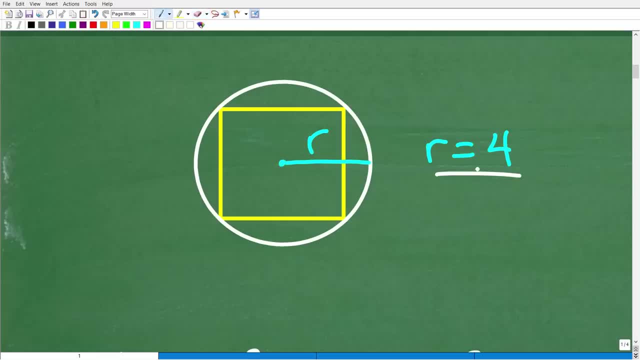 drawing this particular radius from the center out to the edge, and we have a radius of four. So how can we possibly find the area of this, this square, just with this, uh, this information? Well, what we're going to have to do here is take 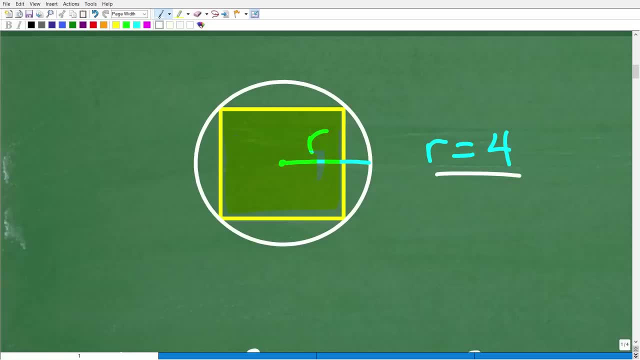 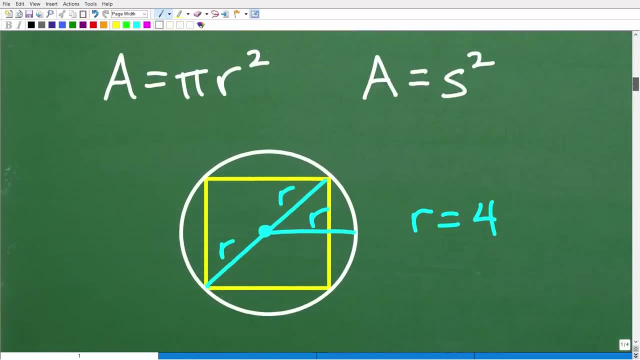 another perspective. We're going to have to look at this problem in a different way. Let's go ahead and take a look at this way right now. Okay, Now some of you might be saying: well, do you know? do I need to know the area of a circle? Well, uh, you, you know, it's not a bad idea to know. 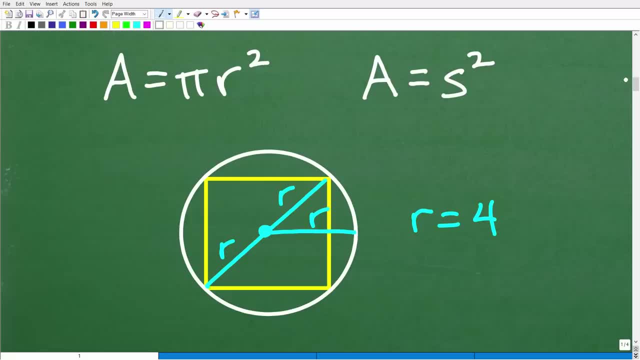 the area of a circle. You certainly- this is a formula that you, should you know, understand, but let me go ahead and just actually tell you what it is. So the area of a circle- just in case you think it's going to help you with this problem- is equal to PI R squared. 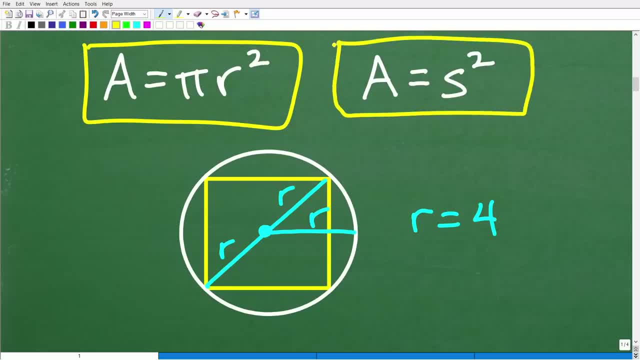 But this formula you're going to need to know. that's the area of a square. So the area of a square is simply the side times the side or side square. right Length times width, uh, or the side square. All right, Now let's get back to this perspective. Uh, you know how can we view this? 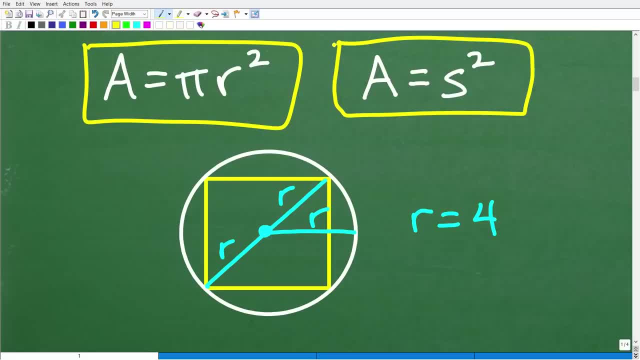 problem uh differently, in such a way that this uh helps us out in terms of getting some more information to understand what to do in this problem. Okay, So let's say we've got, you know the radius of the square. Well, let me just do a quick. 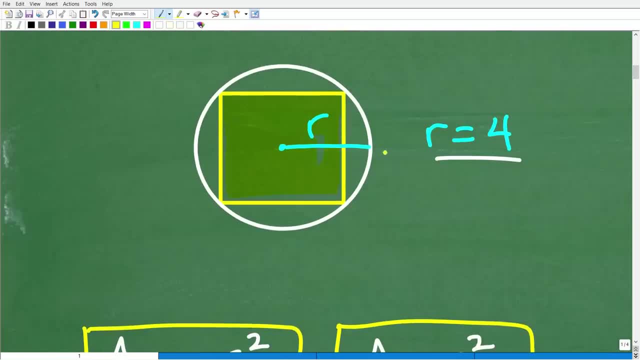 long winded way of saying that. all right, here, I drew the radius this way. this is a little bit of a trick, I'm like: okay, here, here's the radius, it's four. So somebody might be like: 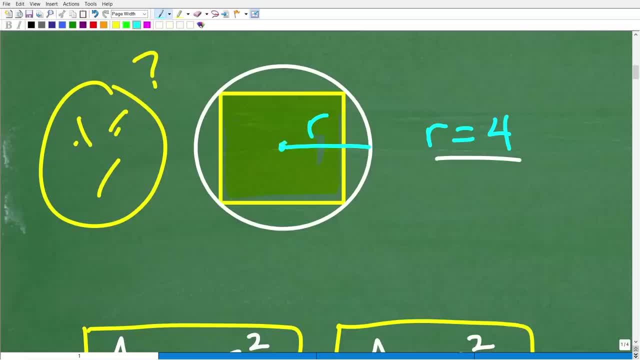 well, I really don't know what to do here because you know I'm trying to get information about the side. Well, if we think of the radius from the center out to the corner, well this is the radius too, And so from here down to this corner of the square is the radius as well. So this changes. 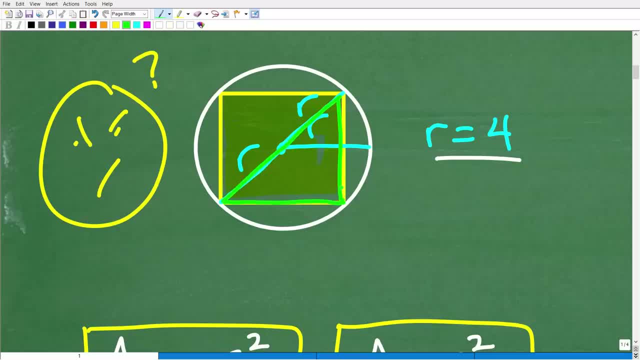 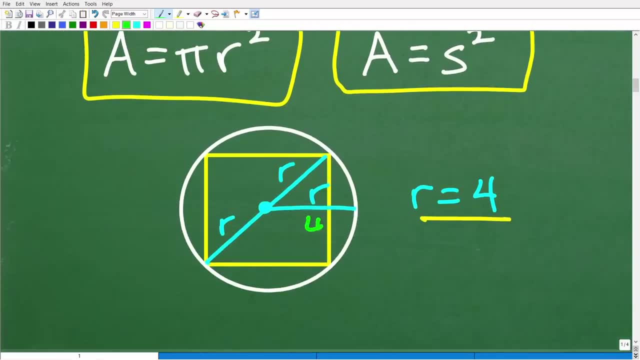 entire length is actually the diagonal of the square, okay, so this is really kind of the secret of doing this problem. so if this is four, okay, well then this is four, right here. and so is this: this is four, so the entire distance of the diagonal, ie this part of this triangle, okay. 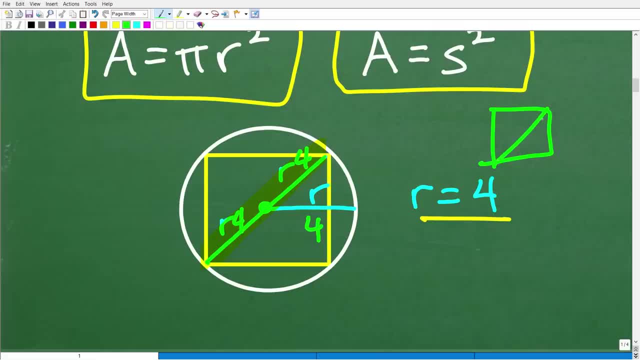 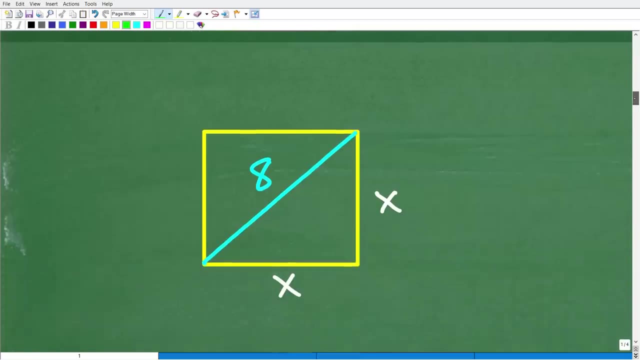 of course we have this square and we draw the diagonal through it. now we have two triangles that are the same, but the the length of this side of this triangle that's called the hypotenuse is eight four plus four, right? so now we can kind of look at our problem in this way, all right? so 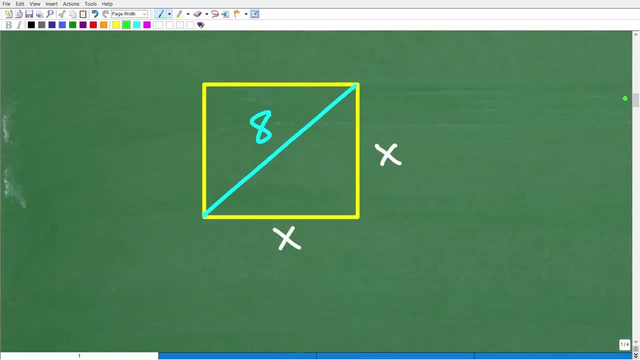 here is our square. we'll kind of get rid of the circle, because now we know that from here, this is the radius, this is four, this is four. so we just kind of now focus in and view the problem in this way. we have this square, and what is the objective here? well, we're trying to find the 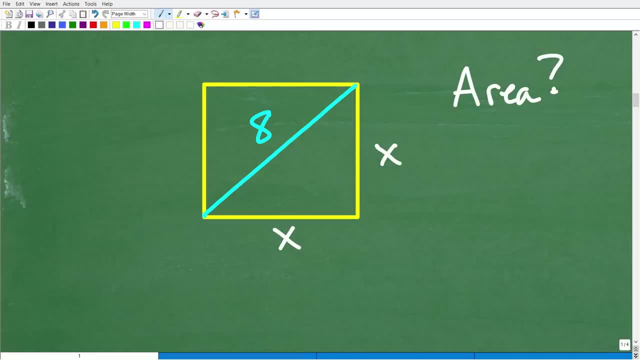 annotation: area of the square. So, just algebraically, what is the area of the square? Well, it would be what It would be this side times this side right, That's the entire area. So the area of the square is simply going to be x squared, But of course we don't have these values for x. So how can we? 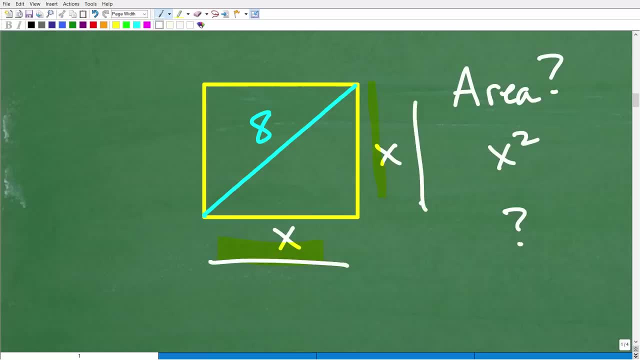 find the lengths of this side and this side, which, of course, are the same side. Well, this is going to be kind of the secret part of this problem- not the secret part, but the interesting part- and you're going to need to know a, one or two formulas. Okay, You can get away with one formula. 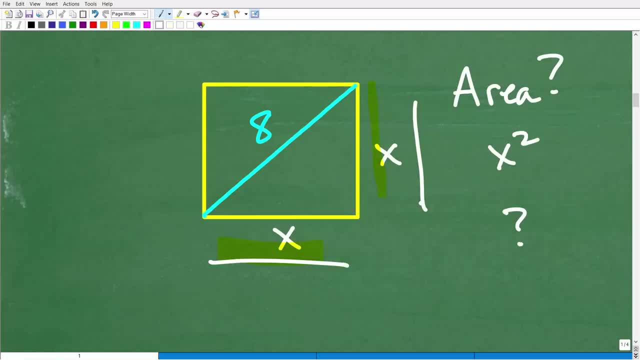 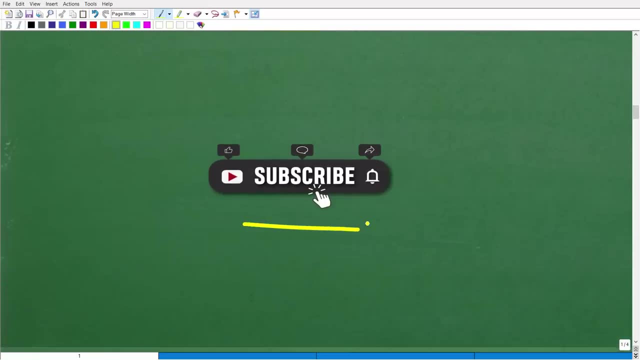 And if you don't remember that formula, then you at least need to know this other formula. You'll see exactly what I'm talking about in just one second, But first I'm going to ask you to subscribe to my channel, If you, you know, if you like this content, you know you might as well go. 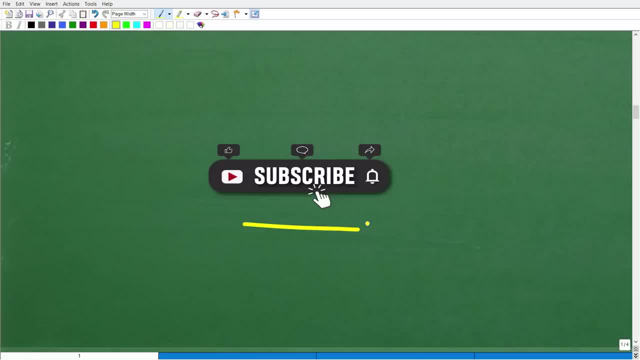 ahead and subscribe. It's a great way to show your support Now for me. you know, when you support me really would you know? I hope you can kind of look at it in a way of supporting other people that need help in math, because by you subscribing it helps that YouTube. 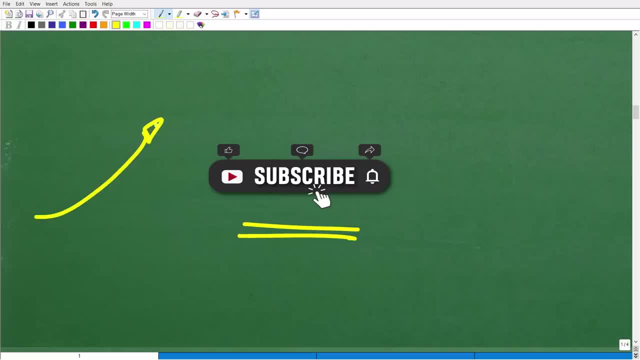 algorithm push my content out to people that are searching for various math topics or just interested in math. it really does help. so if you are going to subscribe, make sure to hit that notification bell as well, and if you're new to my channel- I have about 2,000, actually well over 2,000. 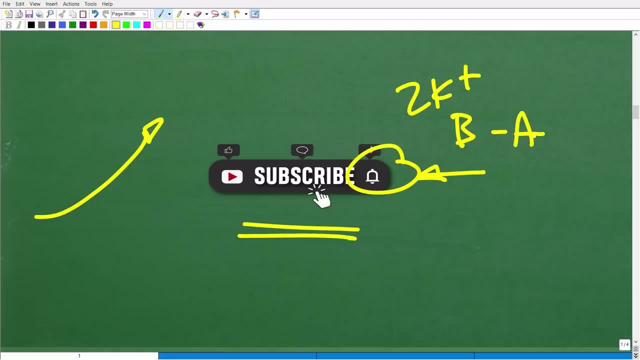 videos from basic math to advanced math and everything in between. so I mean, I kind of go up to calculus on my channel and a lot of arithmetic and of course a lot of algebra, geometry, trigonometry etc. so if you are taking a math course and you know of course with that any one of those particular 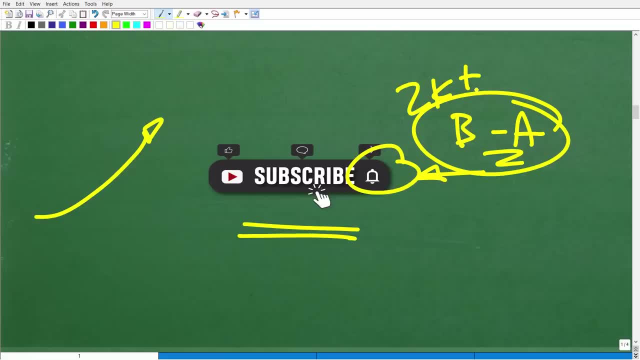 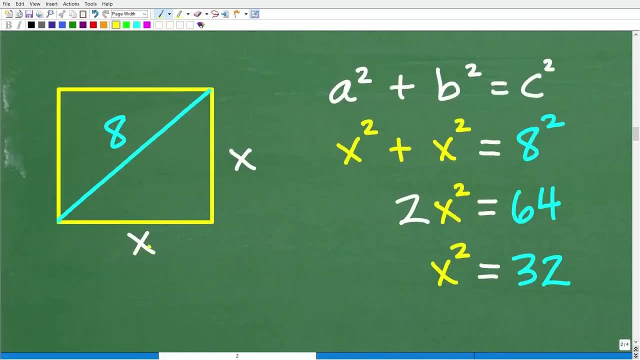 levels. just go through my videos. they're there for you, okay? so let's go ahead and get back to this problem. so now that we understand, all right, well, here is the square x times x is in fact the area, but how can I find what x is equal to? well, you can use one of two functions. 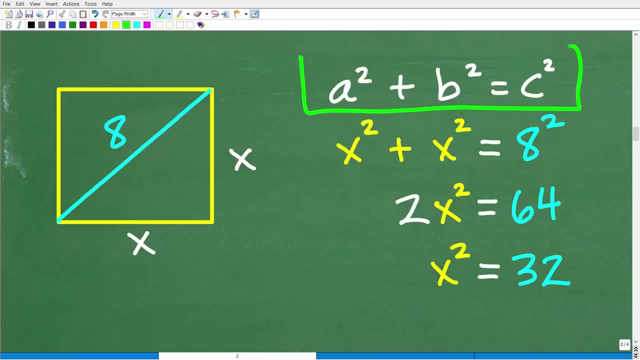 formulas. now, the first formula- and this is the formula that I'm going to use here- is the Pythagorean theorem. okay, and this is a great formula for right triangles. matter of fact, it's probably one of the most important formulas in all of geometry. matter of fact, maybe in all. 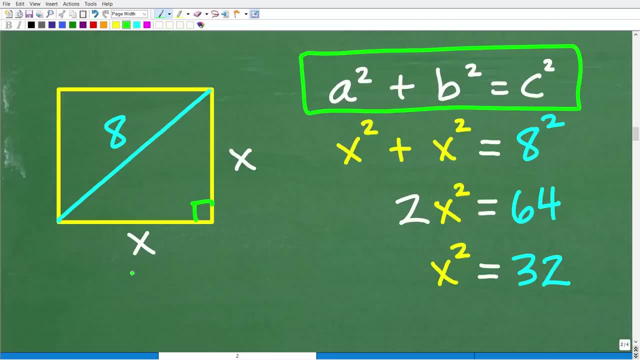 of mathematics. it's pretty simple. the way it works is this: a and b are the smaller sides of a right triangle. now remember: a square has a right angle and the longest side of a right triangle- or longest side, yes, the longest side- of a right triangle, not in all. 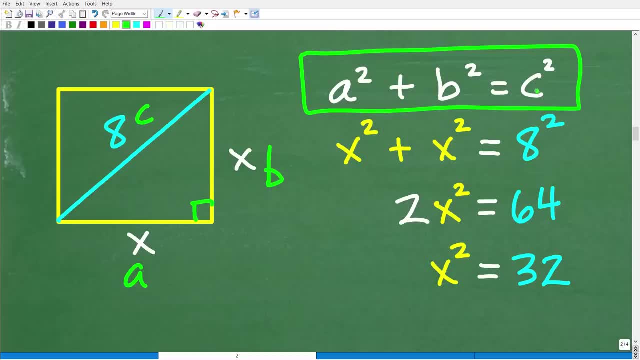 triangles, only for right triangles. it's called a hypotenuse and that's going to always be the variable c. but basically the Pythagorean theorem states this relationship, that the square of this side plus the square of this side will be equal to the square of this side. this is an incredibly 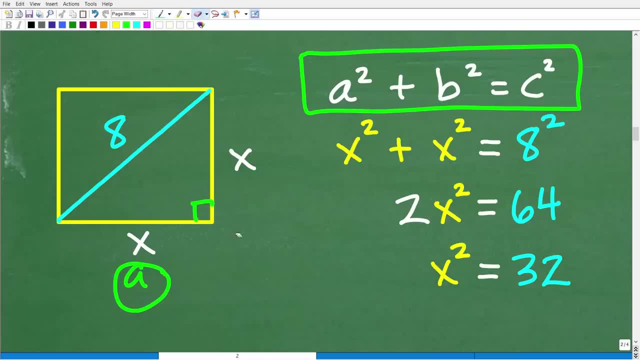 important formula. so this is one approach that we could take to solve for x. okay, now, I'm going to take that in just one second, but let me tell you this formula that you can use. I'm not going to use it here, but this right here, this is a 90 degree angle. 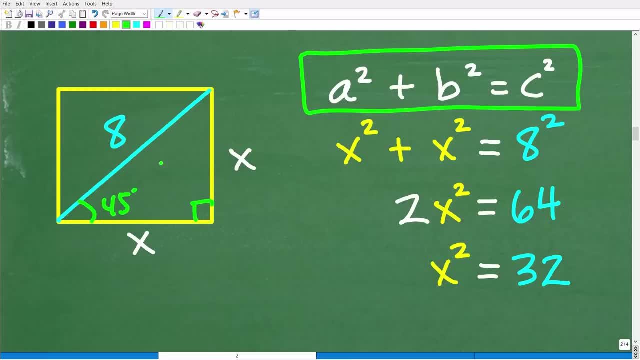 this side's the same, this side's the same. this happens to be 45 degrees and this happens to be 45 degrees, right here. so there is a formula- okay, a special relationship, we call this a special right triangle- that the hypotenuse 8 is equal to this: x times the square root of 2, that's equal to 8. okay, 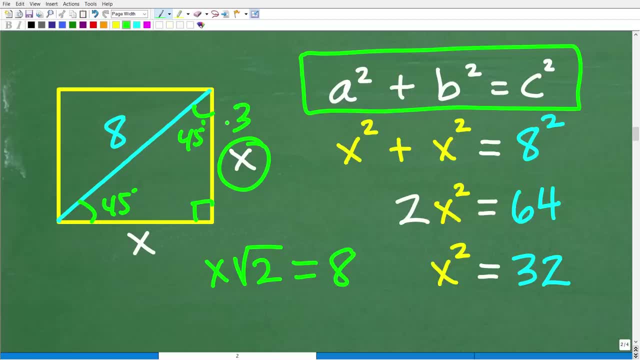 in other words, if I have this side- let's suppose this was 3 and I wanted to express what the hypotenuse, the length of the hypotenuse, is- what you do is just take the side and you multiply it by the square root of 2 and that, in fact, is the length of the hypotenuse. so this is an approach. 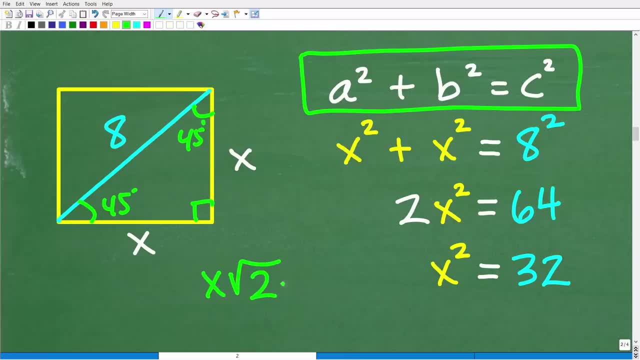 you could take as well. so here, x times the square root of 2 is equal to 8, and maybe some of you were like. you know that's an easy approach to solve for x and it is. however, this is not going to be the quickest way. well, now it could be. it could be pretty quick if you're pretty good. 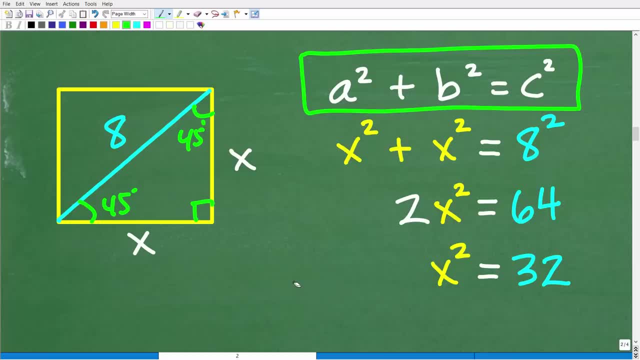 in algebra, but I'm going to go back to the Pythagorean theorem because, remember, are we trying to solve for x? are we trying to find the, the side, what x is equal to? well, yes, we think we do need that, but really we're trying to calculate the area, the area of the square. what is the area? 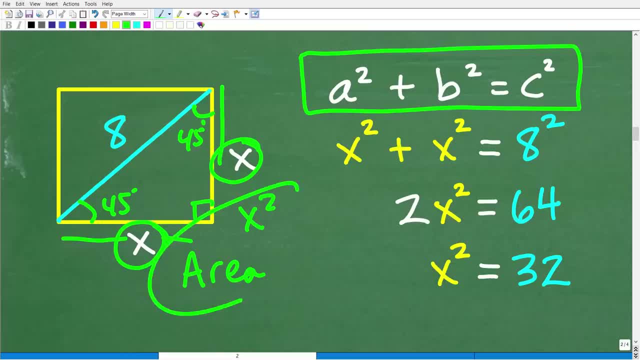 of the square. it's going to be x times x or x squared. this is the answer. okay, so we don't need to solve for x. what we're looking for here is x squared, so let's go and get into it right now. so we have a squared plus b squared is equal to c squared, so a will be it. 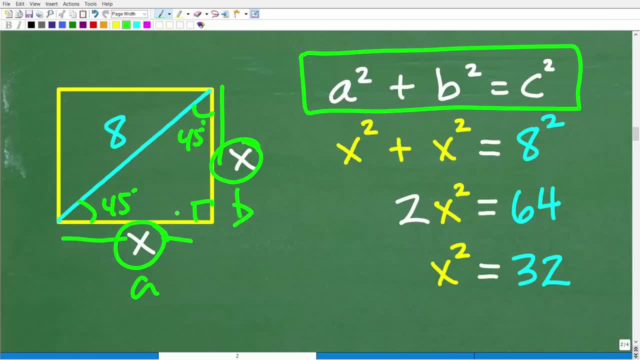 could be this side or this side, so either. of course, these sides are the same. so we'll have x squared, okay, which is same thing as a squared, plus b squared, which, of course, is going to be the same thing, as x squared is equal to c squared. this is the thing that matters the most with the 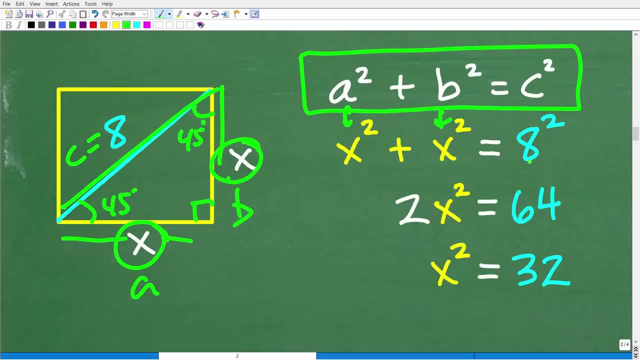 Pythagorean theorem that c is always the highest value of x squared. so we're going to have x squared. hypotenuse, okay. so that's going to be equal to 8 squared, all right. so now let's go ahead and solve for x. but we're really going to. all we need here is x squared, because that is the area. so x squared. 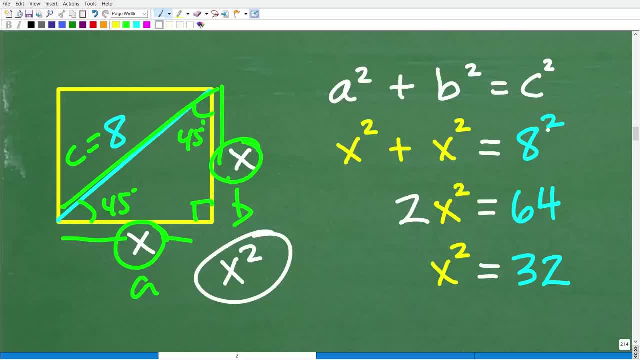 plus x squared is 2x squared, and that's going to be equal to 8 squared, which of course is 64. so to solve for x squared, all I need to do is divide both sides of the equation by 2 and I get: x squared is equal to 32. now a lot of you are going to feel like: wow, I. 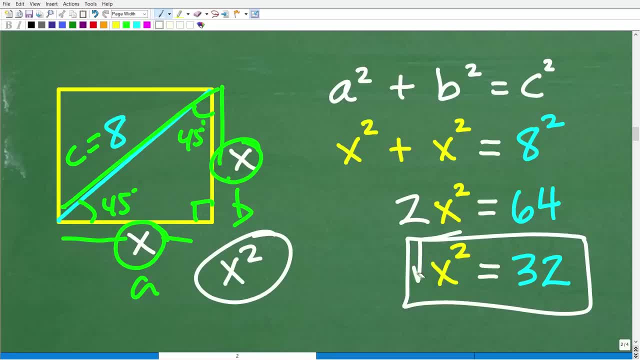 have to solve this quadratic equation by taking a square to both sides. yeah, you certainly can, but you're just going to be kind of going more into, you're going to be taking more steps only to have to return back to x squared, because x squared is, in fact, the area. okay, so again, when? 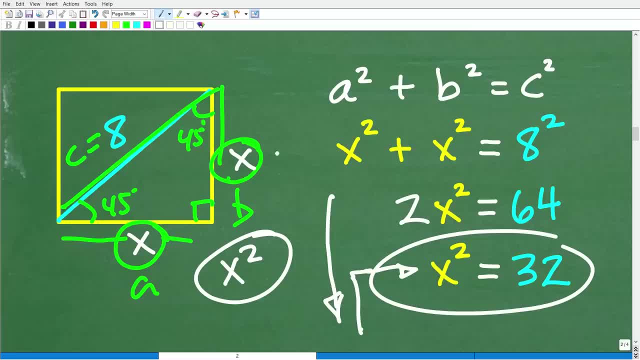 we're talking about area. we're talking about units squared. so in other words, if this was inches, we would have 32 inches squared, okay, so hopefully you found this interesting. this is a great little tool to just kind of emphasize that you need to really be thinking about what a question is. 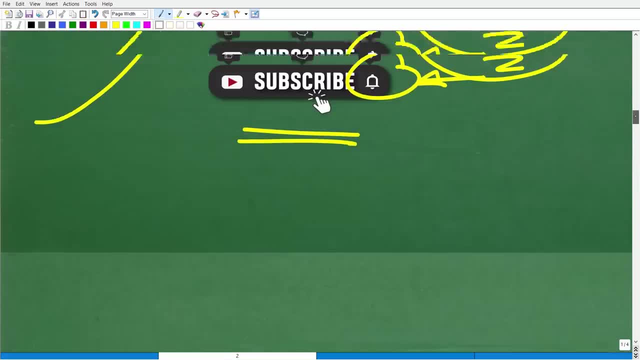 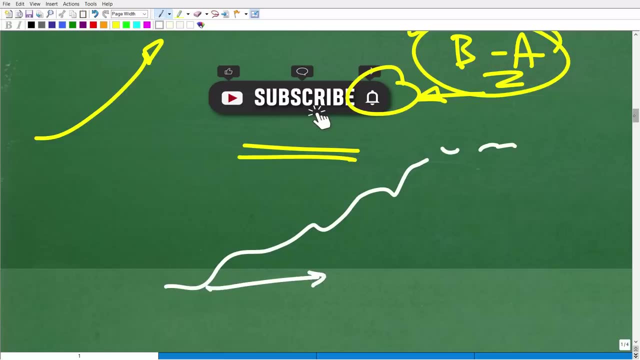 asking because oftentimes we can kind of go off on you know tangents of like you know I need to solve for this, I got to get this and this and that. but you know, really, if you are clear on what the question is asking, you can kind of think about: all right, what is the most direct strategy to 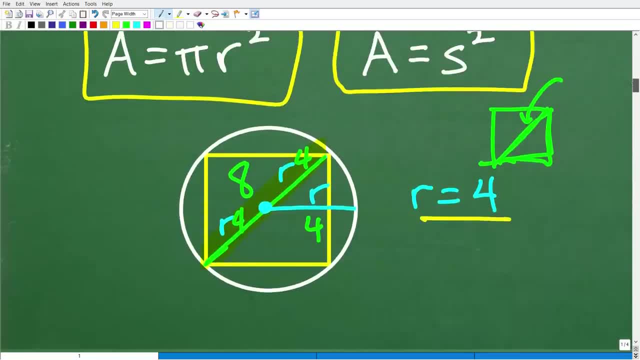 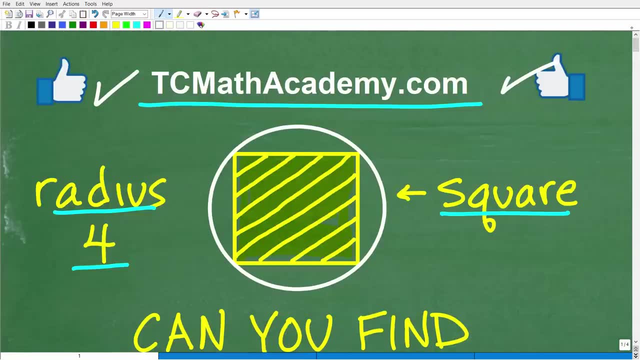 get there. okay, now, if you need help in geometry or algebra, I'm pretty excited to let you know. right now, the time I'm posting this video, I am running a 50 percent off sale off my main courses, which include pre-algebra, algebra 1, geometry, algebra 2 and pre-calculus. this is a once in a. 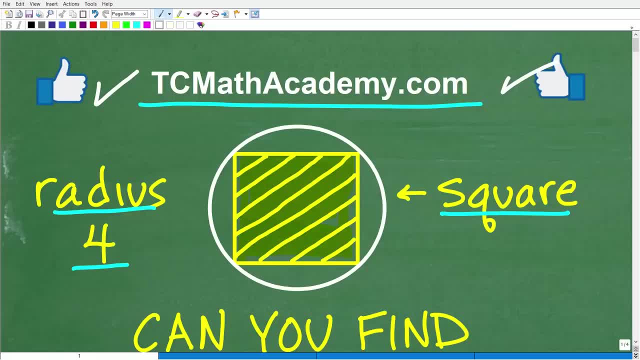 blue moon sale. so if you want to kind of, you know, enroll in one of my courses to really get my best full instruction, well, these are the courses that are for you. so I'm going to leave all the information in the description of this video to include the discount code, but this is going to be.